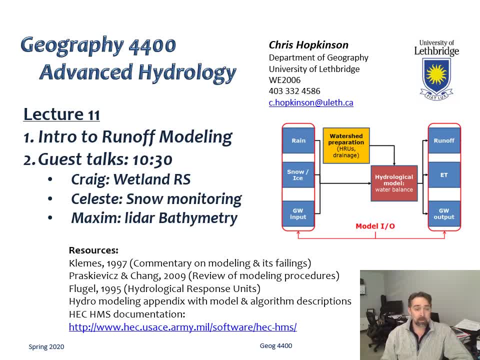 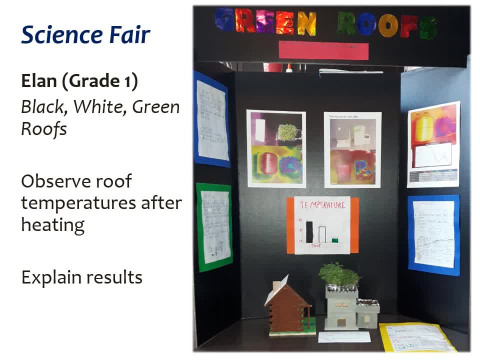 on the materials, You're not going to be evaluated. on the materials, You're not going to be evaluated. types of models, So, from those which are the most similar to the kind of models that we might use in hydrological simulations. So here we see a close-up of 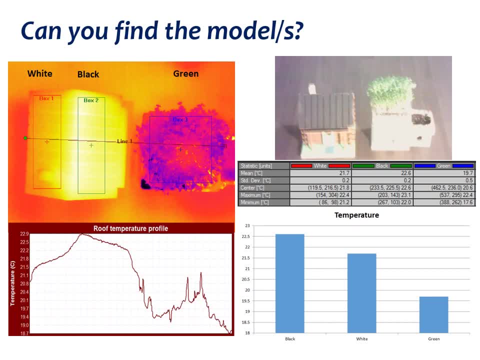 some of those graphics displayed on the poster board, and while nothing you see here represents the kind of phenomena we would typically address in a hydrological simulation, immediately, we find the tables of values, the histogram and the line plot to be familiar data representations that we have encountered. 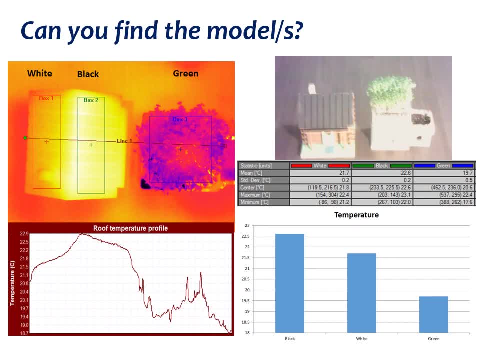 in all of our hydrological labs so far. So the common element here is quantitative or numerical modeling. Now, in this case, the numerical plots we are looking at are, in fact observations or summaries of observed temperature, and so in many ways are more analogous to the kinds of data input we may use in a 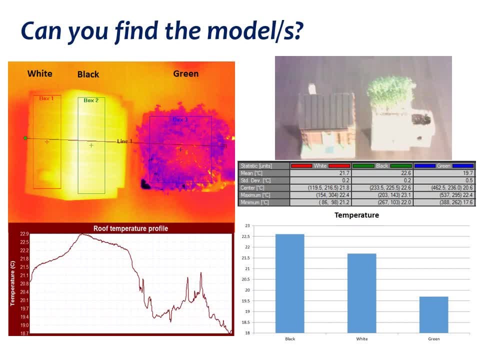 hydrological simulation. However, these numbers are also the result of some behind-the-scenes numerical modeling process, As thermal imaging systems do not directly observe temperature. they record a brightness value That is then converted to surface temperature using a lot of additional information. So, while the numerical processes are different, the conversion 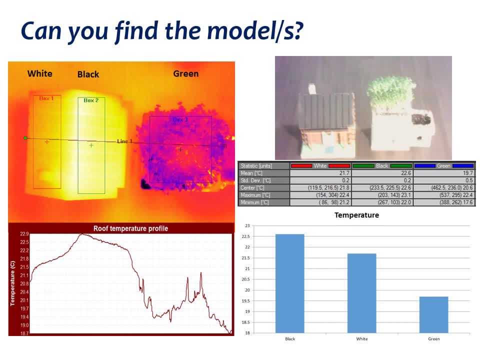 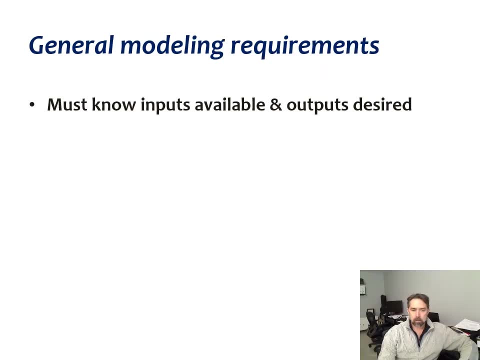 of a brightness value into temperature has some similarity to the conversion of observed rainfall into a modeled runoff output. Now, whether an airfix kit or a global economic forecast, there are common requirements needed in the development of any model: Availability of material data, information and data. 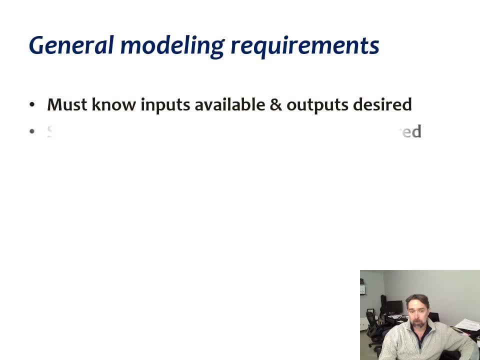 It is important to remember that the model is not simply a simple simulation that can be processed or manipulated. Given the model is a simplification of reality, we must make choices over where to simplify. This may be constrained by input availability or the construction of the model itself. 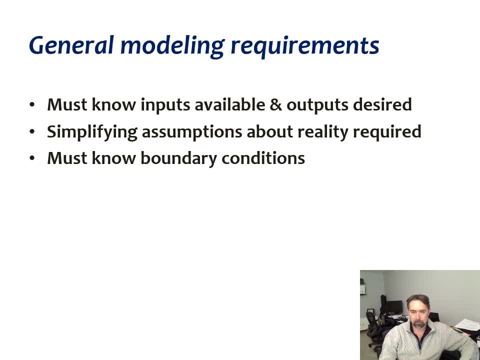 Also for practical earthly purposes. we can assume reality is unbounded in space and time. Models, however, do not appear out of thin air and they can only represent a finite spatio-temporal domain. Consequently, constructing a model or may require some blending or extension beyond the edges of the domain of interest. 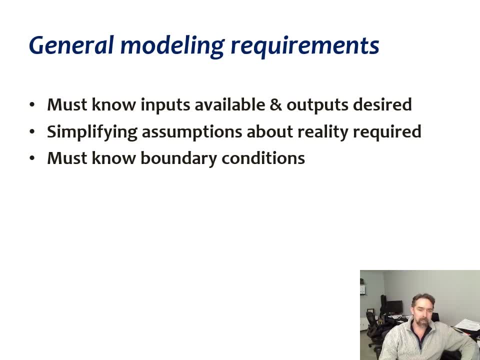 to enhance the model realism, and this is known as defining our boundary conditions. Models usually have a particular purpose, and when used or applied outside the intended domain, their usefulness breaks down. So now, in your own time, consider these modeling requirements and try. 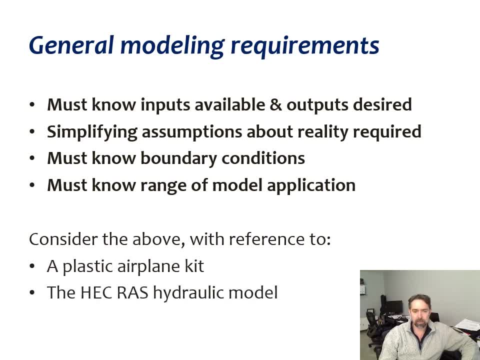 to apply the previous examples of an airfix plastic kit or to the HECRAS hydraulic model that we've looked at previously. So we'll look at those over the next two slides. Okay, so this is where we would normally have a group five where you'd all go off and 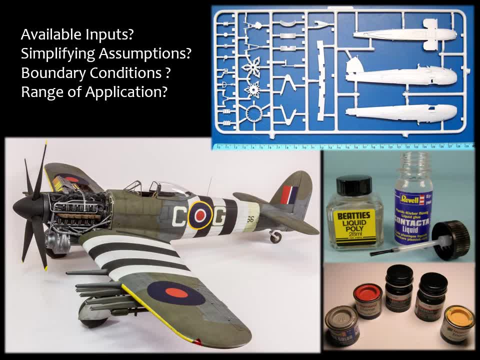 into your groups, have a discussion and then report back to the class. But instead let's just look at what we have on the slide here. We've got some plastic mold with components of the model. We have a finished model of an airplane. This is our airfix kit, and then we have some glues and 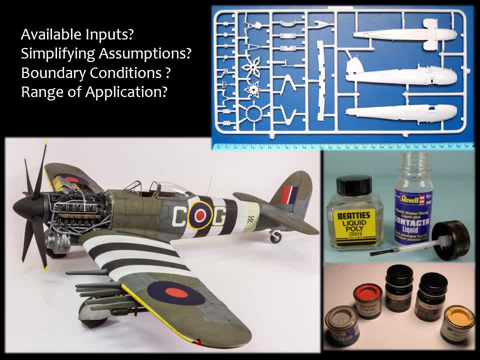 some plastic. So we've got some plastic molds with components of the model. We have a finished model of a glues and paint pots there. So, given this, what are our available inputs into this model? What are some of the simplifying assumptions, What are some of the boundary conditions And 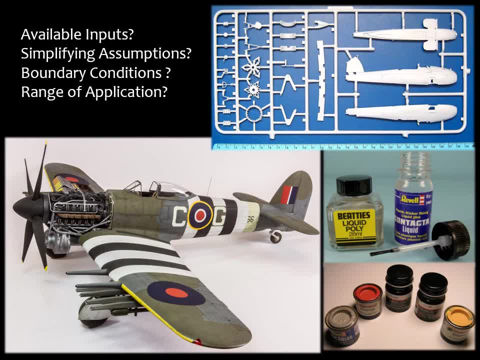 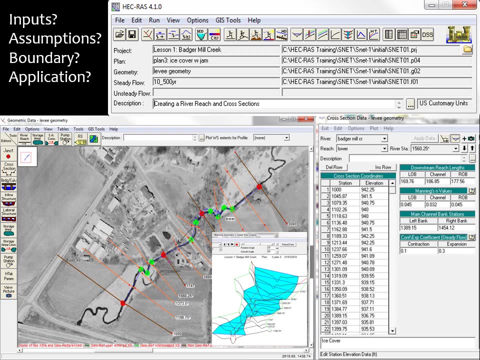 what's the range of application? So I'd like you to spend a little time now thinking about that and if we have the opportunity, we'll discuss. Okay. so now the same exercise again, but now with the HECRAS: water level modeling environment. So available inputs, simplifying. 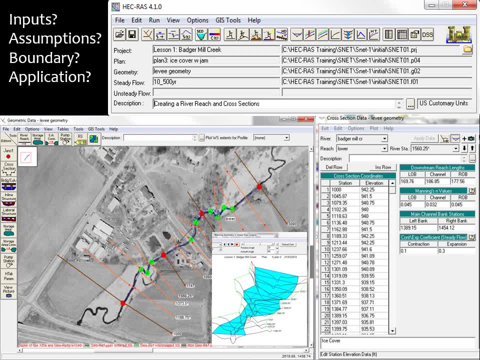 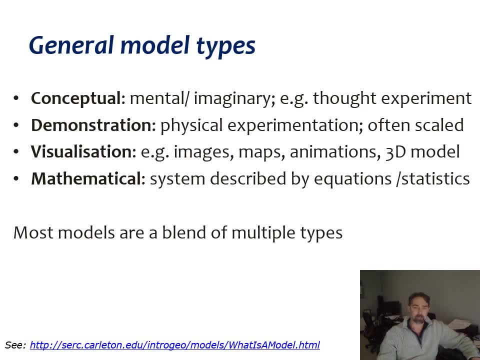 assumptions, boundary conditions, range of application. Now that we have looked at some of the general model examples and considered some basic requirements, let's define some general classes or types of models. If you Google model classifications, you'll find many different types. 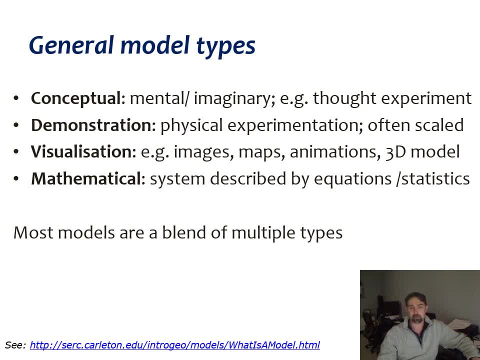 However, most models can generally be said to fall primarily into one of the above classes, though models can also belong to more than one of these classes. A conceptual model helps us understand some aspects of reality or their interactions. Any form of modeling effectively requires a 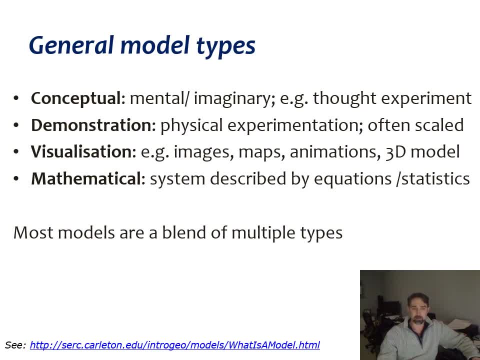 conceptual model as a first step. A demonstration model is an act of doing something to otherwise simulate or describe reality. It could be a lab experiment, such as when using a scaled flume to study wave action. All visualizations, whether one, two, three or four-dimensional, are a model. 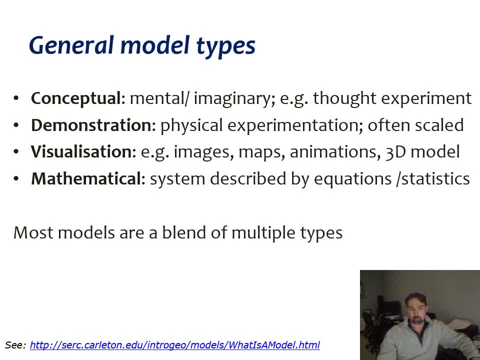 of something or some event. In hydrology, we are mostly concerned with mathematical models which can be considered as a model of something or some event. In hydrology, we are mostly concerned with mathematical models which can be considered as a model of something or some event In 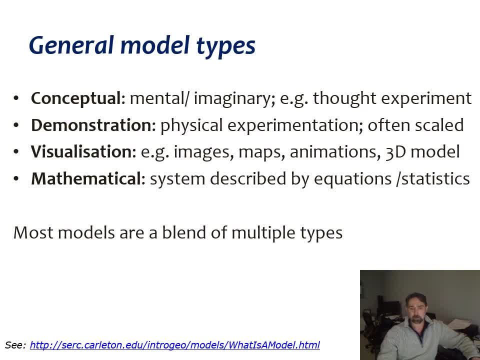 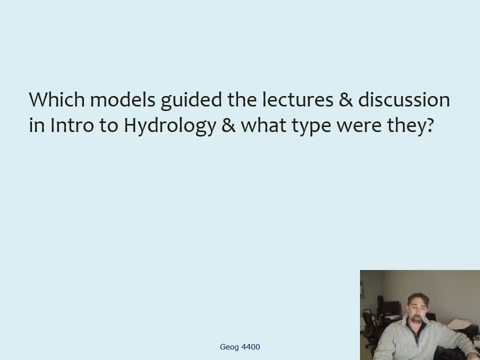 rane. models can be equation or statistically based, though in most models, even hydrological, are a blend of multiple different types. So if you think back to our introduction to hydrology lectures, we may not have explicitly discussed hydrological modeling, but can you think of any models that guided our discussion? In particular, there was one model. 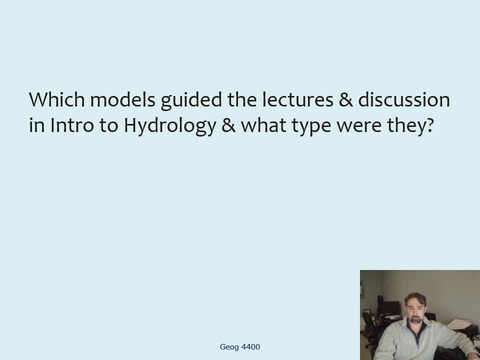 that referred to throughout the course. Well, all the model types noted were used in lectures and labs, but conceptual models were used for several of them. In practice, there was a model that and mathematical constructions of the hydrological cycle and water balance were the building blocks. 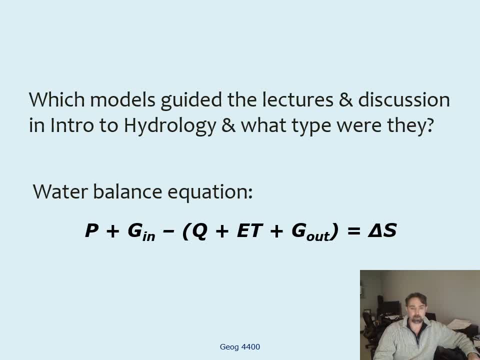 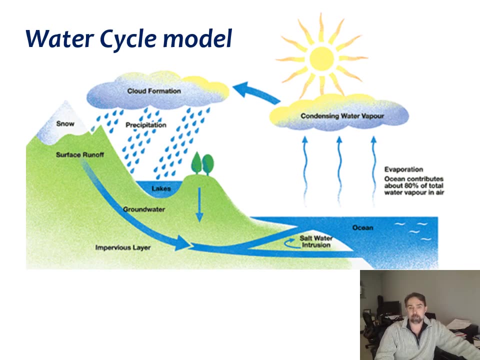 of all material presented. In particular, the water balance equation was presented as a simple mathematical model representation of the Earth's water cycle. And of course here we have a visual or illustrative model of the water cycle, which is itself a conceptual model of the Earth's. 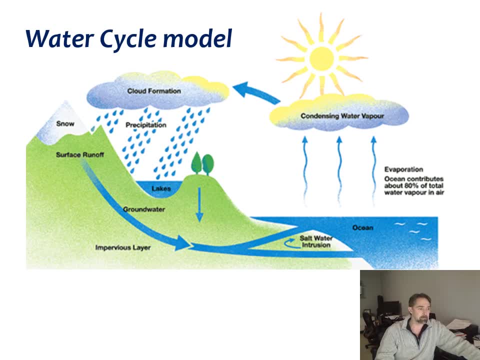 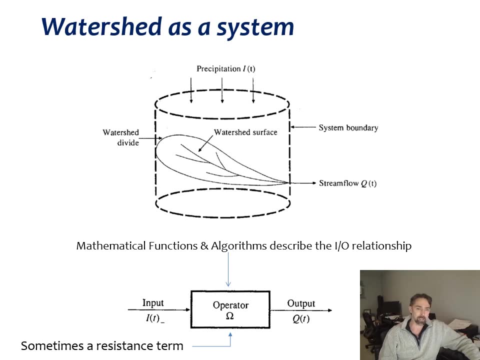 hydrological system. So, as was introduced in Introduction to Hydrology, the basic unit in hydrology and hydrological calculations is often the watershed. So at the top of this slide we see a conceptual graphical model illustrating hydrological inputs of precipitation and outputs of runoff, all bounded by the extent of the watershed. Below this we see a systems diagram. 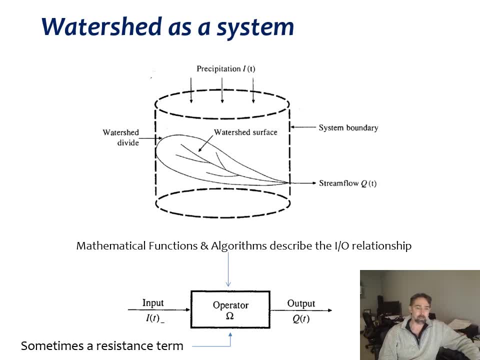 that could be used to represent the same processes whereby some mathematical algorithm or resistance term relates the precipitation input to the runoff output. You may recall the unit hydrograph as such an example. Consequently, many hydrological models concentrate on relating inputs to outputs. within the spatial extent of a watershed, The 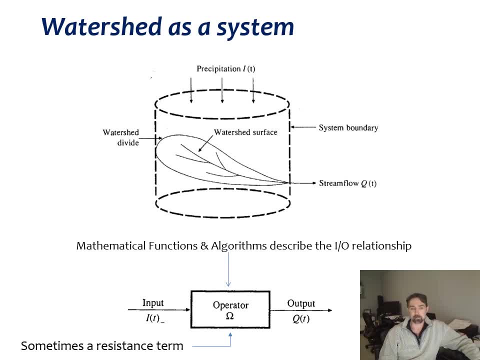 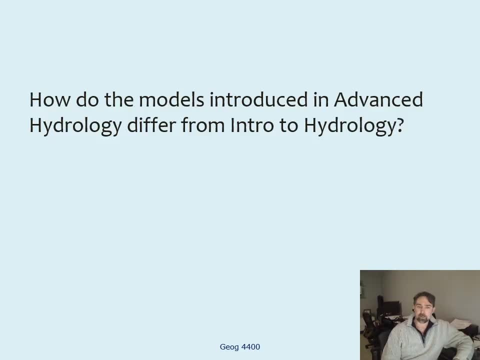 nature of the mathematical description of these relationships can be very simple or highly complex. So if all models are some variation on the watershed water balance that we know in the past, how do the models introduced in advanced hydrology differ from intro to hydrology? 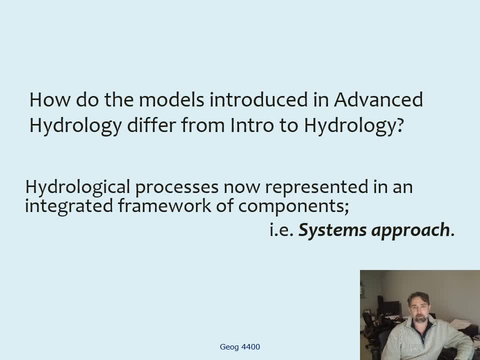 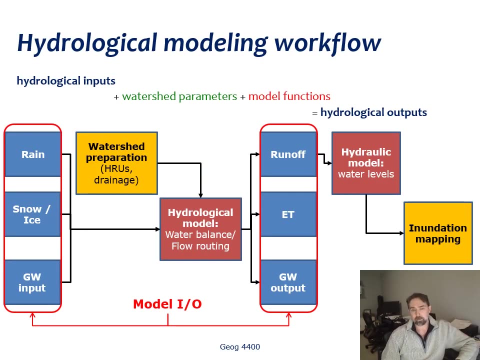 Well, basically it's because hydrological processes are now represented in an integrated framework of components, which we can refer to as a systems approach. Here we see a conceptual visualization model of how we have dealt with hydrological principles in the advanced hydrology course so far. In this conceptualization we see the linkage. 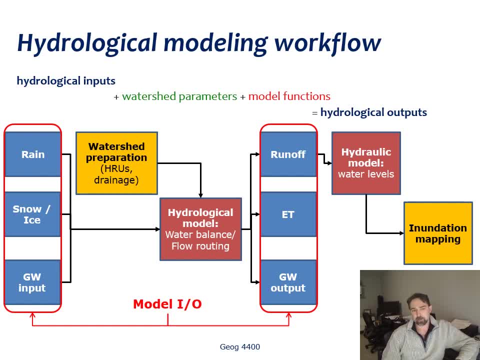 between outputs of one model component and the inputs of another. For example, lab 1 dealt with elements of the far left input side of the overall model, while lab 2 addressed the design phase of a hydrometric study to obtain basic input and. 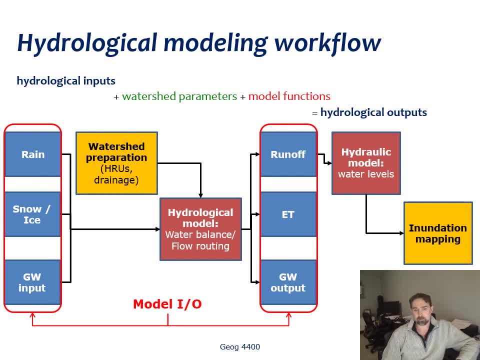 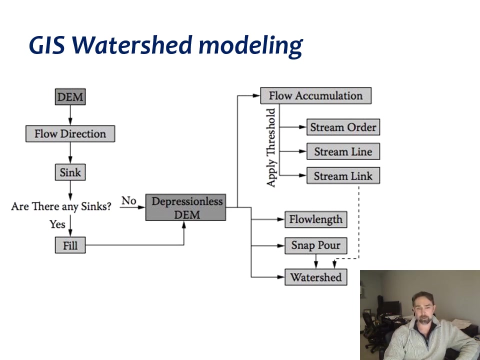 output data. Lab 3 developed watershed or floodplain parameterization skills, whilst the team project examined floodplain and nodation components of the modeling workflow, And so hopefully, with this diagram, you can see how all of the components fit together. Similarly, any individual model component, such as the watershed extend and flow routing. 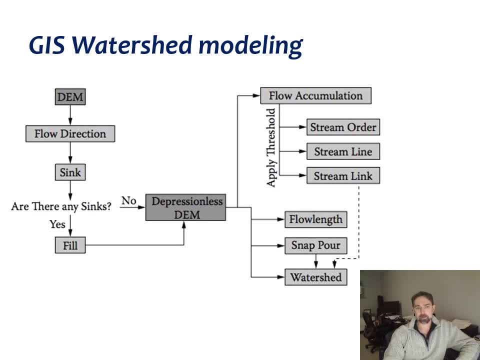 components can also be subdivided into constituent elements. Here we see a standard GIS process that you should all be familiar with by now. I'm sure you can all recognize this as the watershed delineation workflow, which is itself an example of a modeling process. 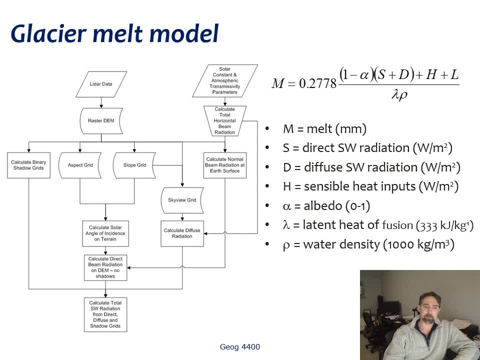 And here we have yet another GIS routine to serve as an example, This time an energy-balanced snow or ice melt model. Here, each term in the melt equation is represented by raster surfaces which are updated periodically through time As long as the basic terrain grids are available. 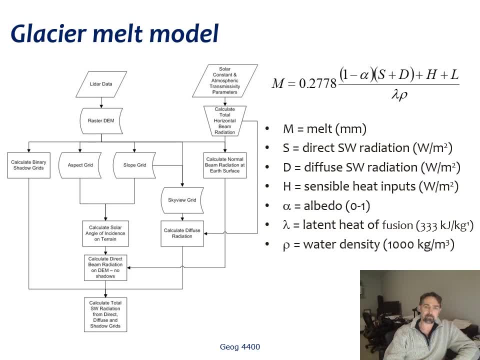 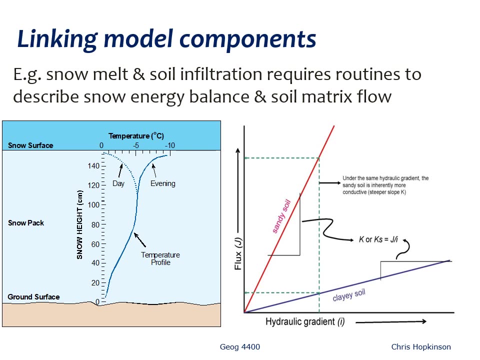 such an energy-balanced model is relatively easy to construct and run. However, this model will only estimate melt. It will not estimate flow routing. We will look at flow routing shortly. What happens at all? the model component link points, ie the lines connecting the boxes in. 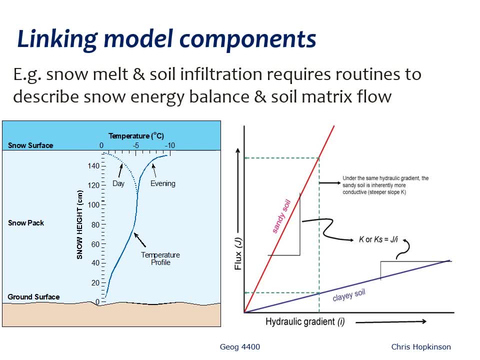 these flow diagrams. This represents the real complexity, as at one level, it is fairly straightforward to imagine which model components pass to which, Such as an energy input will drive snowmelt, or water that is infiltrated to soil will contribute to groundwater. I won't. 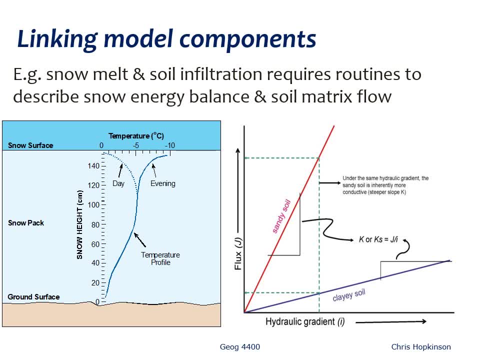 get into detail to this, but within most Hydrological models each component is its own mini-model or subsystem where the input output willene toidez on. So, more specifically, when any of the models that are showing fully integrated snow melt or layers correctly, any oncoming unit outs today is subject to a horizontal verlation ratio to net water intake. For examples, put two thousand without explore those three other objectives, Well as toppings and similar olic blocks keeping out your flow- diagrмотр gum dreams- you will realize that snow litter is in between theabbotie. 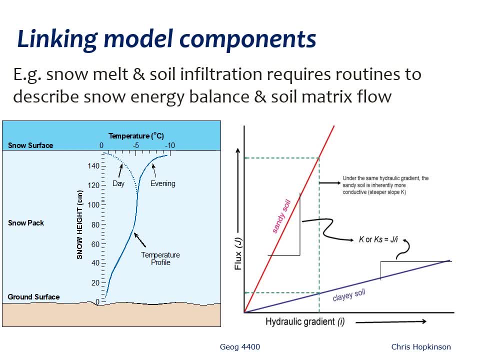 and storage. In the cases here we might take energy and mass inputs to calculate a bulk snowpack mass and temperature profile. As the snow heats up, it eventually melts and loses mass as melt water. This mass of water will be transferred to the next possible node in the model framework. 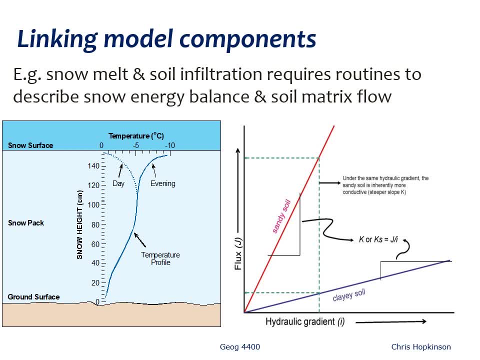 This could be the soil zone, which is also its own temporary storage system, with a unique set of parameters that will control infiltration and through flow of water. The model, components and transfers could be very simple or very complex, depending on data availability and what we know. 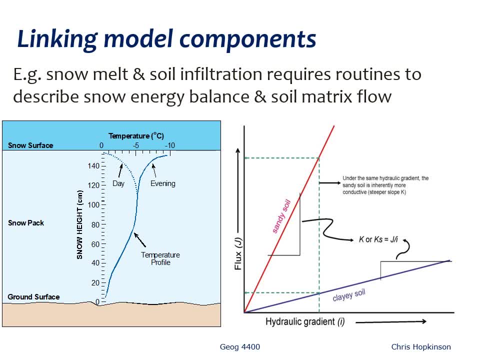 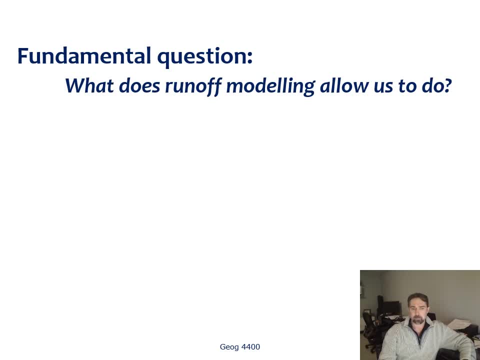 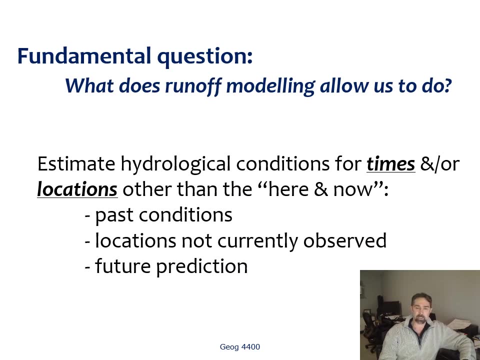 about the system being modeled. So complex hydrological models generally require a systems approach. but what do these models actually allow us to do? As humans, we want to make decisions about where we put ourselves or our region. We want to make decisions about where we put our 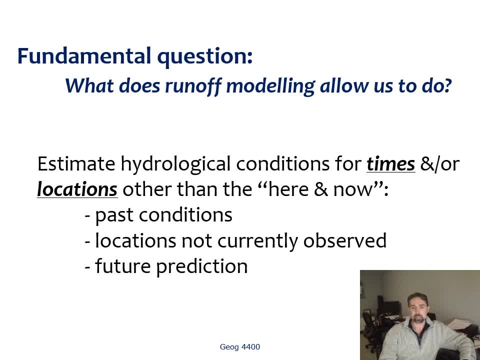 resources, based on the best possible information concerning either the availability of water resources or the avoidance of water hazards. Water is a very dynamic medium, so what it is doing today is not a great indicator of past or future conditions. Models allow us to fill these gaps in our observational data, either in time or space. 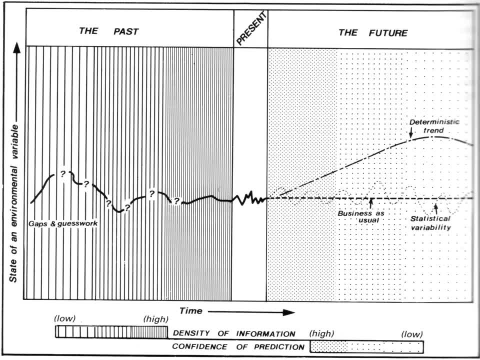 For example, we may have observed fairly steady fluctuations in the recent data record, but if any of these gaps are observed, we may have observed a significant increase in water balance. If any elements in the system we're interested in are gradually changing, such as with climate change or land use, then we can't expect water balance or runoff behavior to 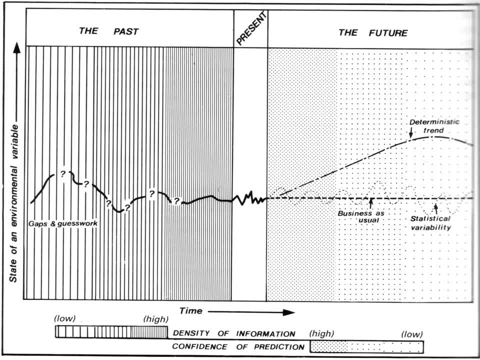 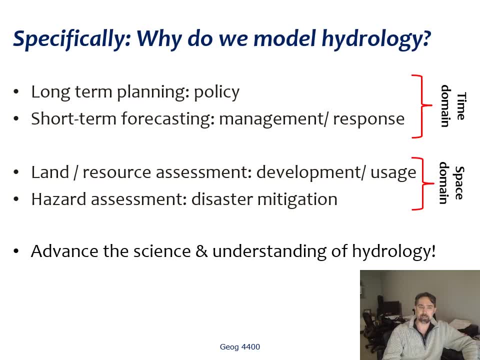 remain the same. More specifically, then, our needs for hydrological modeling address time-dependent planning and management needs, as well as to define the boundaries on spatial development and hazard mitigation measures. And, of course, such models can also be used to satisfy our scientific curiosity about hydrological processes. 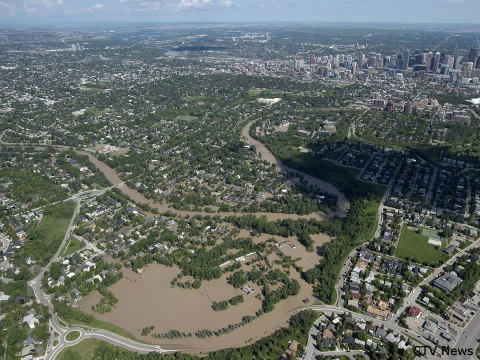 And as examples here are two water-related hazards that we may wish to mitigate through the simulation of either the temporal likelihood of occurrence, eg probability of a flood in any given year, or the spatial extent over which the hazard will occur. The first example is the Calgary. 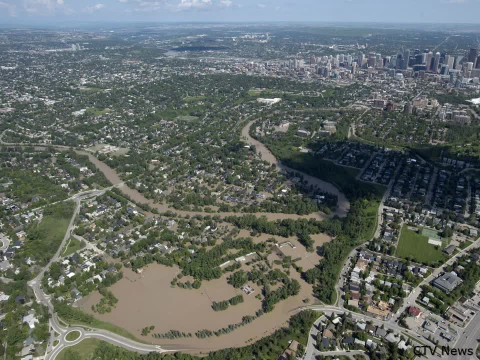 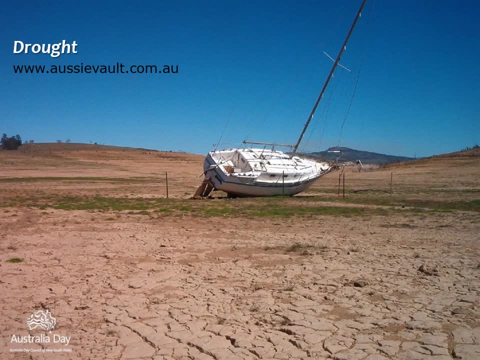 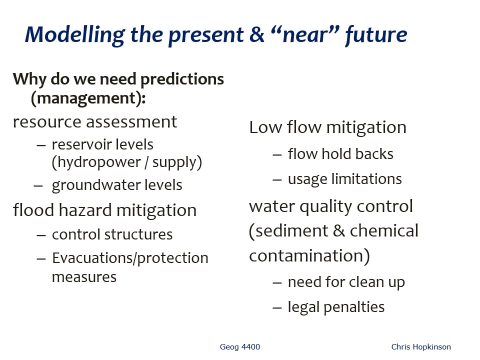 Flood on the Bow River in 2013.. And the second shows a stranded boat in a dried-up reservoir at a stretch of land during a prolonged drought. Many tasks, then, require fairly constant monitoring and short-term prediction in hydrology. Here are some application examples of 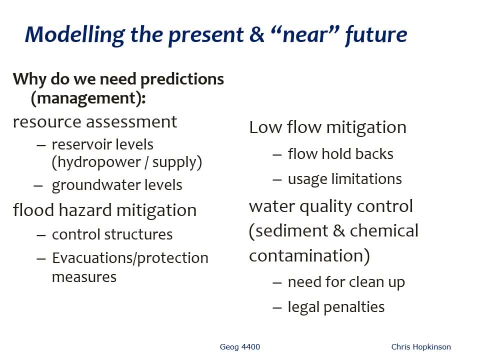 short-term flow forecasting needs. Most of these will fall into the category of management, as they support real-time decision-making processes During a potential flooding event, for example, the emergency management services will watch the river flow forecasts frequently, as this might inform on decisions on flow. 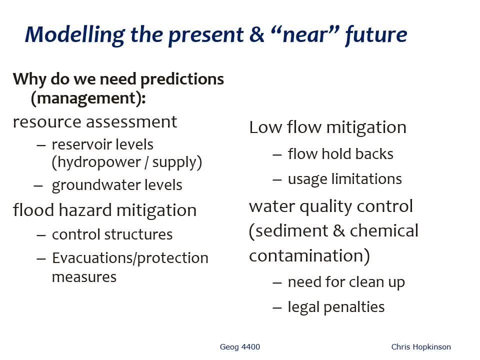 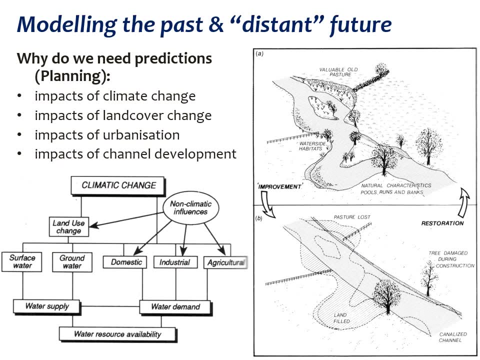 holdbacks or releases, temporary flood plain defences or on evacuation orders Where land cover, land use or climatic influences have changed over time and are expected to continue to do so, then we need long-term simulations for planning and policy purposes. Changes in glacier cover and melt at sentry scale. 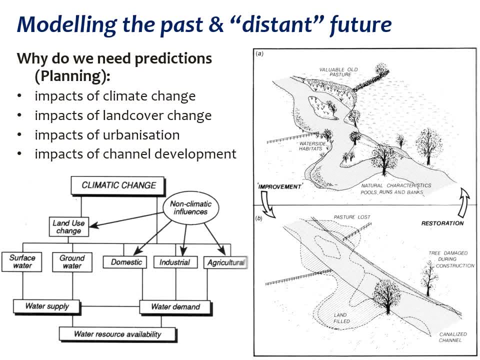 is a situation where provincial governments need predictions to be made at decadal to sentry scale to inform on water allocation rights. At a municipal scale, simulations can be performed to understand the long-term flow or water quality impacts of flood plain development, channelization or even flood plain restoration projects When setting 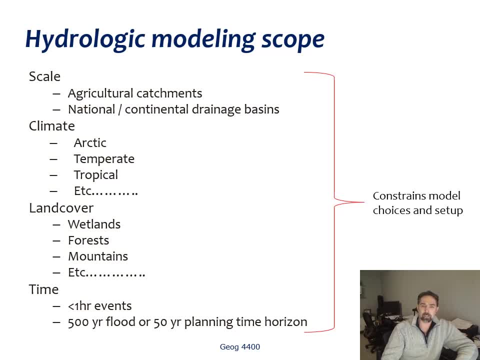 up or choosing a model, it is essential to consider the modeling context, ie for what environment, time period and over what area are the results needed? Sensible decisions over model choice and data requirements cannot be made unless this is clear. For example, will we need 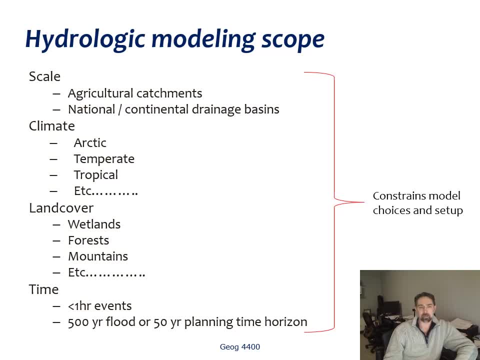 to model at the scale of an agricultural catchment or across an entire continent. Are we dealing with Arctic or tropical climates or somewhere in between? Do we have one dominant land cover or many, And do our simulations need to be made at a high resolution time step such as one hour or over many centuries, where even 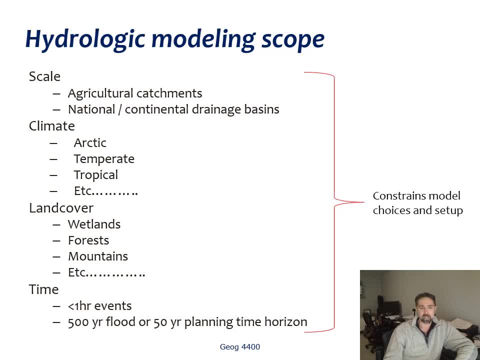 an annual time step may be too fine-grained. Answering these questions will place constraints on the technical and operational requirements of the model, the type of model we need and how we set it up to get the job done. The intent of any hydrological model, of course, is to represent the processes. 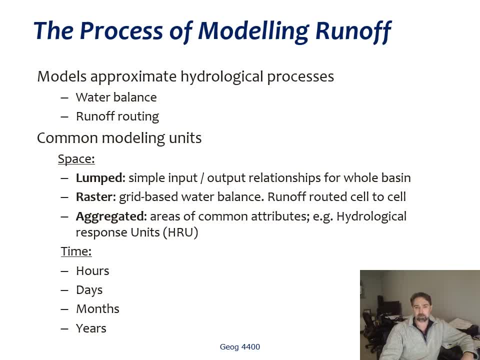 occurring in the environment. This can be simple or complex, but there are two fundamental quantities that need to be considered. The first is the volume or mass of water entering and leaving. each of the model sub- components is typically estimated using a water balance approach. 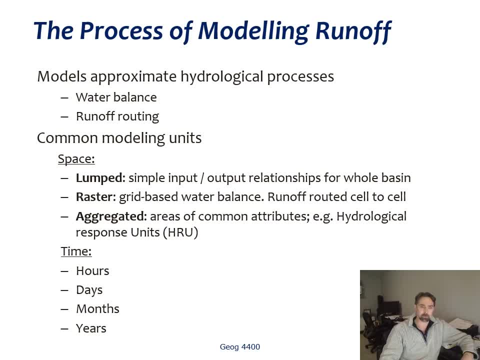 And the second is the timing, or transfer of water from one model component to another usually requires some form of flow routing. The manner in which these quantities are estimated depends on the space and time of interest and the data that are available to support the simulation. As such, most models will tend to have a 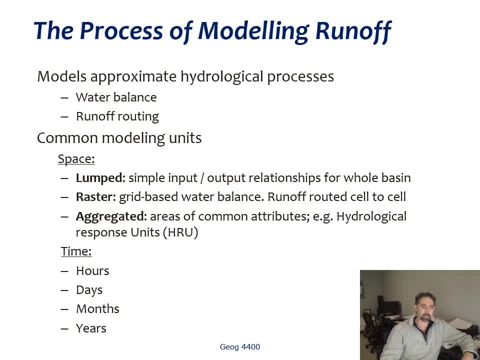 fundamental spatial and temporal unit over which calculations are performed. Here we see some examples. In a spatial context, we can either adopt data inputs, outputs and calculations that represent the entire drainage area of interest, which are known as lumped, or we can distribute our data and calculations through space. 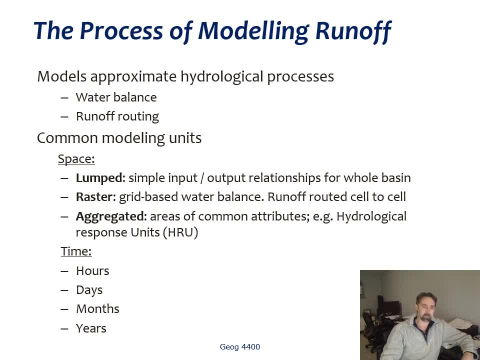 using either some uniform raster representation of the land surface or an intermediate form of landscape aggregation. Similarly, we can adopt high or low resolution, time series, data and calculation steps, which will be constrained by data availability and the time step that best captures the processes that need to be. 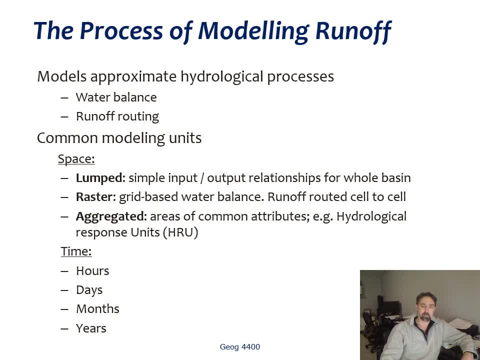 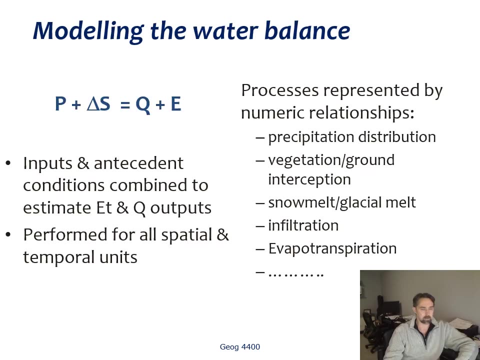 simulated in order to obtain credible results. For example, floods occur over short periods and will need a higher resolution time step than evaluating either the impact of long-term glacial ice to water resources or the influence of drought on crop production. So here we have our old friend, the water balance equation- again A water balance. 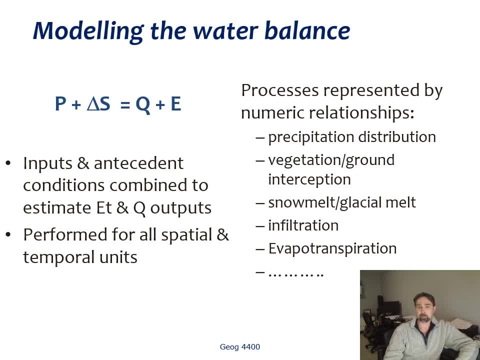 is usually calculated for each time step and spatial unit within the modeling environment. All the major processes that we have discussed in the Intro to Hydrology course, some of which are listed here, can be simulated as part of the overall modeling exercise. But whether they are, 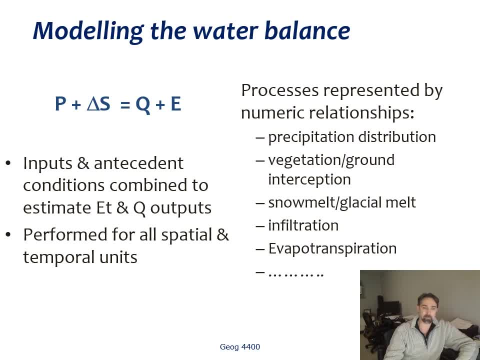 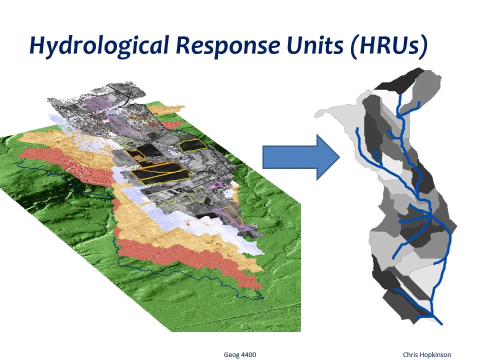 simulated or not depends on data availability and the needs of the model. The water balance can be calculated for an entire watershed or over a grid or aggregated areas such as hydrological response units. Okay, so just what is an HRU or a hydrological response unit? 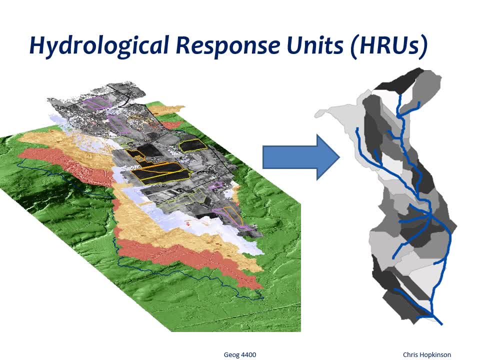 To get a more complete answer, please refer to Flugel's paper that accompanies this lecture. But in a nutshell, HRUs are useful as they represent aggregations of land surface areas that have common attributes, such as infiltration, albedo, roughness. 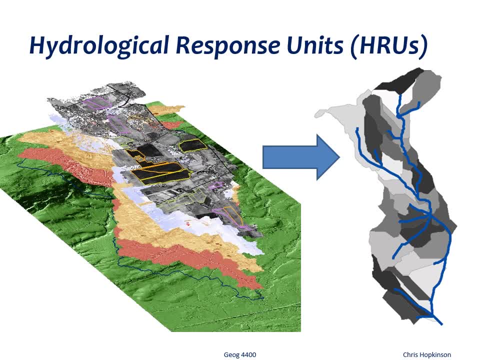 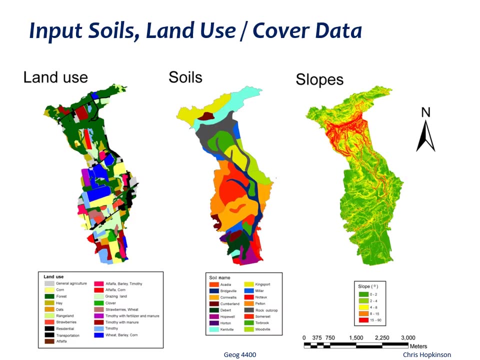 land cover, etc. This allows model parameters to be assigned to a handful of land surface units instead of every single grid cell, and thus improves model computation efficiency. So, as you can imagine, this is typically a GIS process, And here we see some examples of input land surface attribute layers. 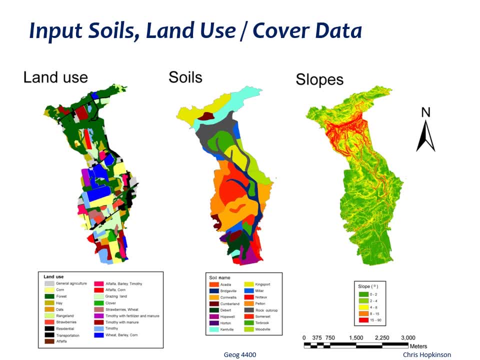 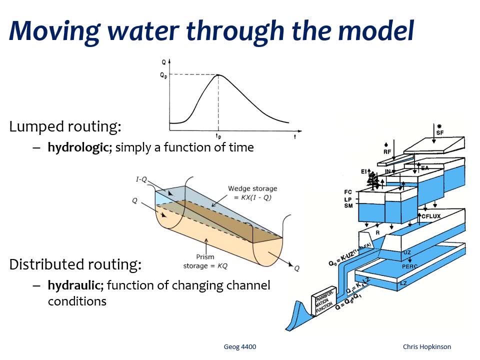 that can be combined to form HRUs representing common land cover, soil and terrain attributes. Once the water balance has been calculated for land surface model components, the water needs to be transferred to the next step within the model. Routing can be from water storage to storage or as runoff within a channel. 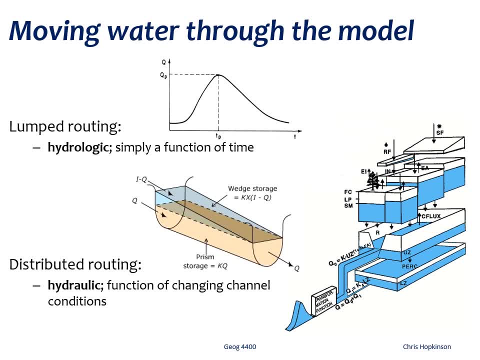 system, which is also a form of storage, as any flow entering the channel system must take time to reach the channel end point of interest. We won't discuss methods of flow routing here, but one common approach uses linear reservoirs that are represented by recession constants, which slow down the transfer of flow from one storage to the next. 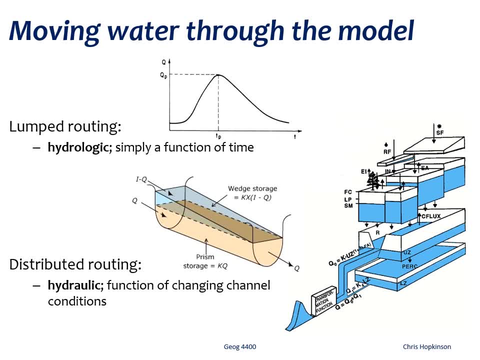 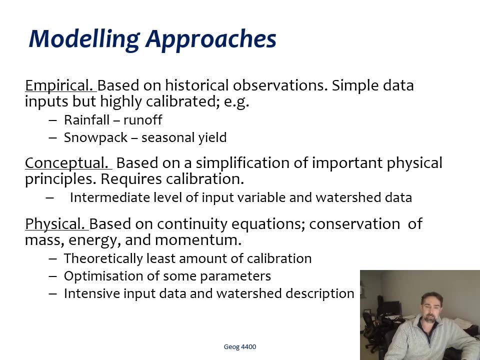 throughout the model using a sequence of recession equations. Another popular approach is Muskingum routing, which models flow in a channel as a function of wedge storage along the river reach. Okay, now we know the basic processes of hydrological modeling, let's consider the broad categories of models that are out there. 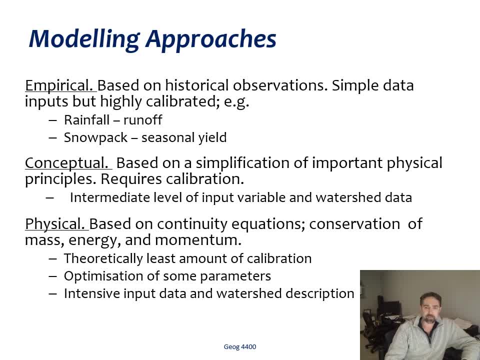 It should be clear that not all environments or modeling needs are the same and data availabilities in different locations are widely different. Here we see three modeling approaches based on their data and calibration needs. Empirical models are highly calibrated as they predict runoff response based on 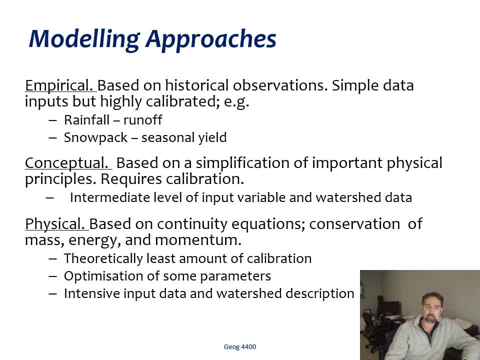 historical precedence. Such models are of limited value in a drainage basin that is experiencing changes to its hydroclimatology or land surface attributes through time. Conceptual hydrological models tend to focus on a small number or maybe one dominant watershed or hydrological process. 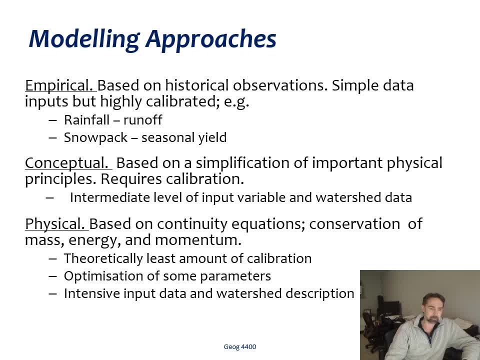 and thus tend to be limited in their application domain. Physical hydrological models use the principles and mathematics of physics, leaning heavily on continuity equations and conservation laws. In theory, then, such models can be executed with the least amount of calibration, but on the flip side, such models can be 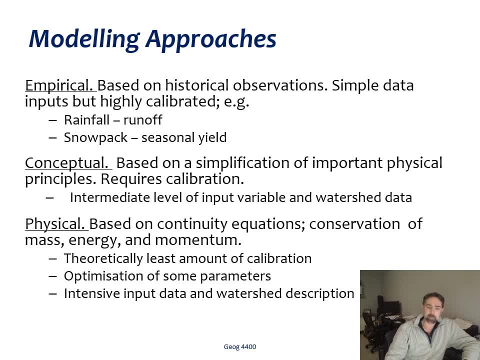 extreme consumers of data, both in describing energy and mass inputs to the system and in terms of describing the watershed system through which water must pass. If we perform detailed scenario testing or make long-term forecasts under conditions of a changing environment, then which of these modeling approaches do you think we need to adopt? 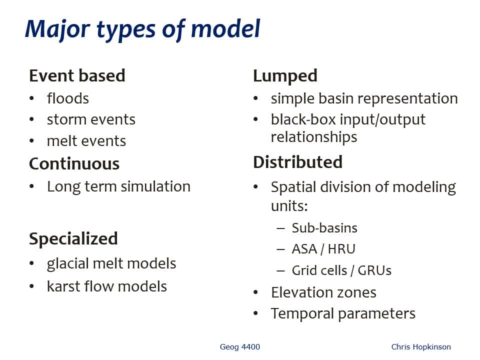 It should be clear that models come in many different forms, and here is another list of the ways by which we can stratify model types. On the left, we see a roughly temporal stratification into event and continuous models, as well as an acknowledgement that there are 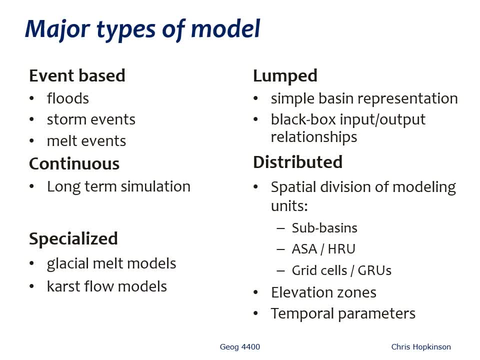 specialized models that may not fit into the traditional models. For example, glacial melt models may require a dedicated modeling framework, as surface runoff from a glacier may not adhere to the typically adopted terrain-based rules of surface water flow. that assumes water tends to accumulate downslope. 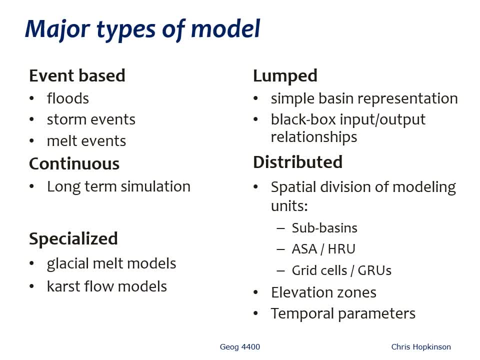 Similarly, karst environments possess surface sinkholes, bypass flows and the possibility of subterranean flow pressurization. that cannot be handled in traditional watershed models. To the right, we see spatial models of the surface runoff from a glacier. We see spatial stratifications into lumped parameter. 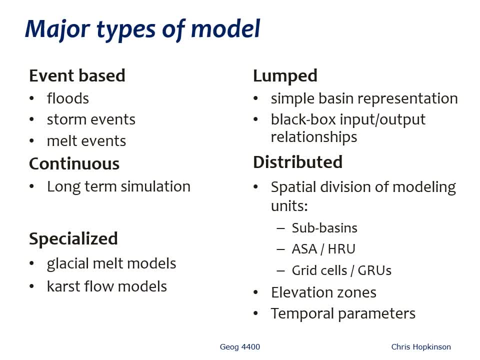 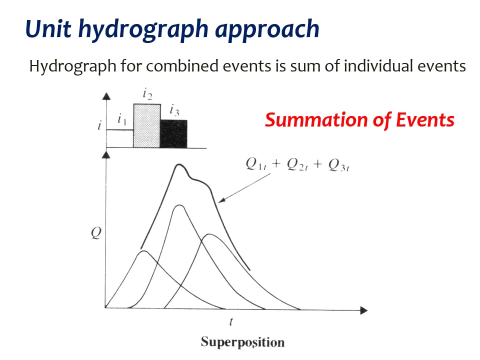 or simple input-output models and various forms of distributed parameter models. We have already noted raster and HRU distributions, but other popular forms of spatial model distributions are by elevation, sub-basin or even by distance from the basin endpoint. The next four slides illustrate specific model types of gradually increasing. 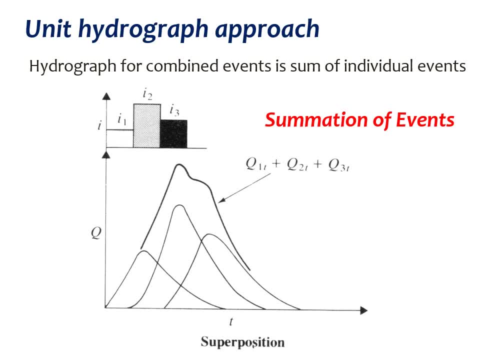 sophistication, distribution and physical representation of real-world processes. The first example is the empirically calibrated and lumped parameter unit hydrograph approach for simulating runoff at a specific river location for a given upstream rainfall amount over time. The unit hydrograph approach makes many simplifying assumptions about the 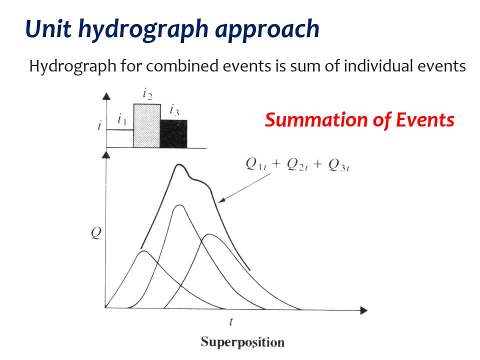 relationship between rainfall and runoff, such that a downstream hydrograph can be estimated by applying a scale factor and time lag to each unit, eg one inch or one centimeter. Within this simple framework, each unit of rainfall through time can be simply scaled up to generate a. 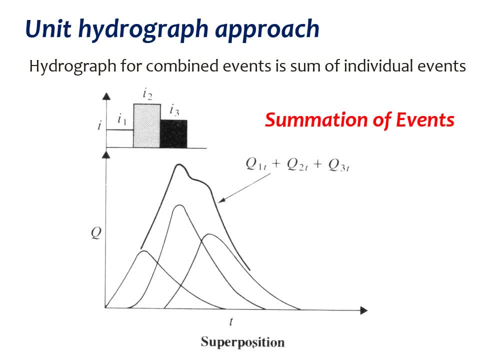 complete event hydrograph. Such an approach must be calibrated for a given area using many years of data. While this can be useful to estimate approximate runoff yields and durations for specific events, this approach is not appropriate for long-term simulations or in situations where antecedent conditions or the watershed properties 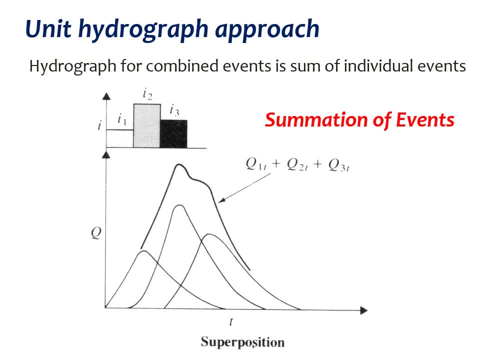 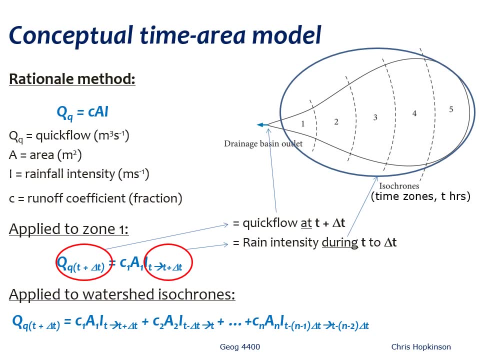 immediately prior to the event can vary widely. This next example is still a lumped parameter approach that requires calibration, but now we see some space-time distribution in the modeling steps. The rational method is a conceptual time-area model that ignores process detail and simply. 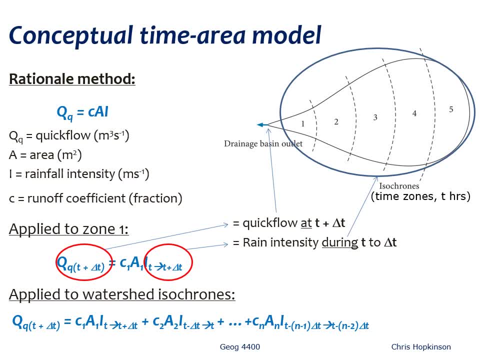 models, water balance and runoff behavior as a function of isochrones or contours of time. The model assumes that rainfall within a given zone upstream of the basin outlet will incur a predetermined amount of loss and will be reduced. In this example, we can see that the rainfall in the basin outlet is 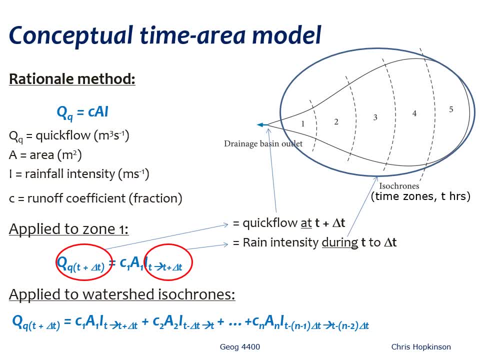 retarded by a certain amount on its way to that basin. endpoint Discharge is a function of the area over which rain falls, the intensity of the rainfall and the loss or runoff coefficient over each region of the watershed. It's fairly easy to calculate, but only 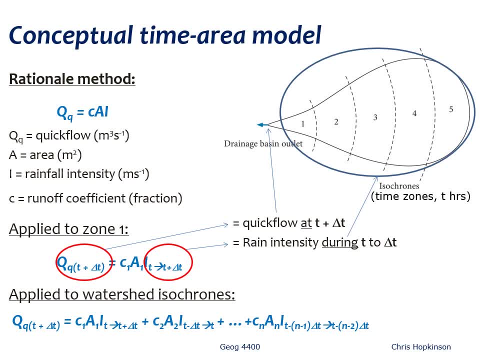 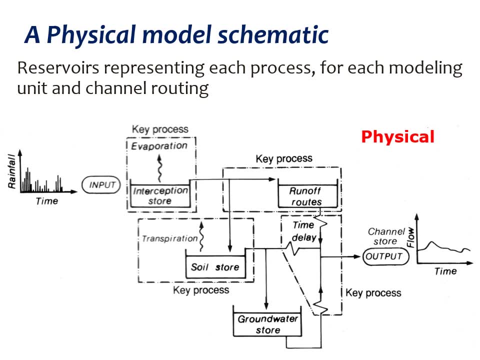 of limited use in practice. As the antecedent conditions can change, so will the runoff coefficient. So here we see, our first physically based hydrological modeling framework, where key processes of precipitation, interception, evaporation and infiltration to soil and groundwater are treated explicitly. However, while there is physical realism in this, 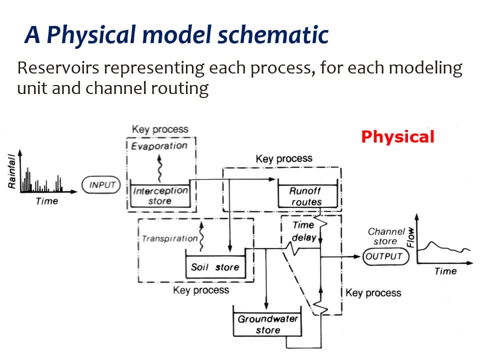 type of model framework and there is some distribution of flow components amongst watershed storages and flow pathways. this is still a lumped model because there is no spatial distribution. Instead, we see a cascade of mathematical reservoirs from precipitation input to runoff output that represents the watershed as a whole. 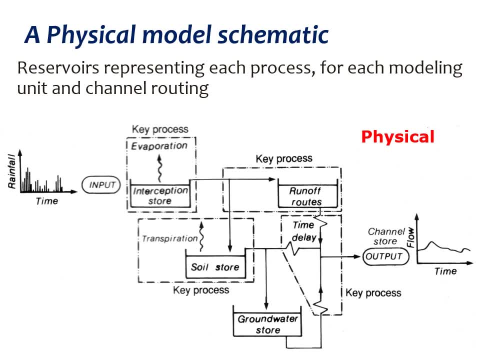 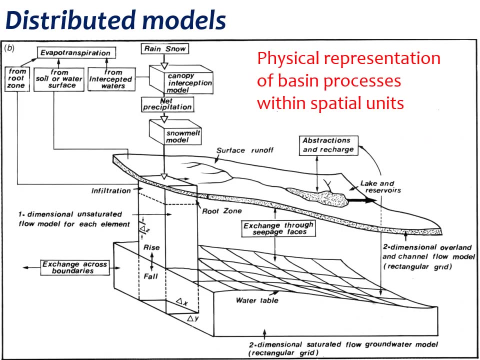 Such an approach may be adequate for small watersheds or in situations of fairly homogeneous land surface attributes with minimal variation in seasonal antecedent conditions, but will tend to perform poorly over larger and more complex regions or over very long time scales. And so here we arrive at a fully physical and spatially distributed model framework. 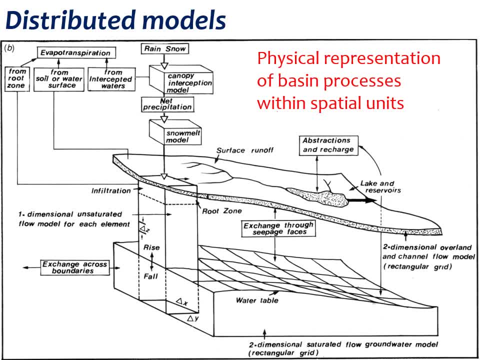 As with the last framework, we see a similar treatment of water balance components, but now we also see the associated calculations are performed for individual grid cells across the land surface. Clearly this is a much more realistic modeling approach that has the opportunity to better represent important hydrological processes. 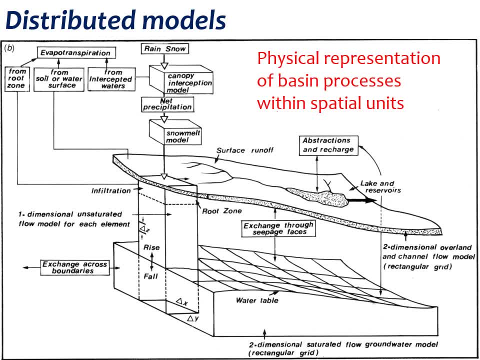 But, as noted earlier, such approaches can be data intensive and computationally intensive and therefore require an understanding of the watershed environment that is not readily available, And this can also require that many assumptions need to be made. Consequently, the advantages of embedding spatially explicit process realism: 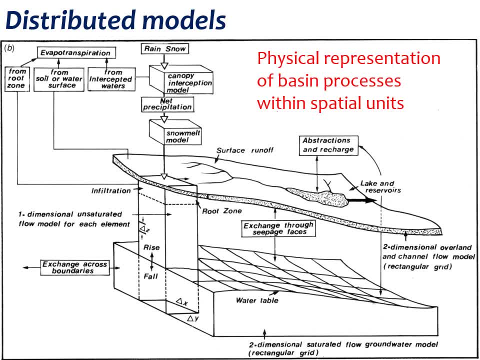 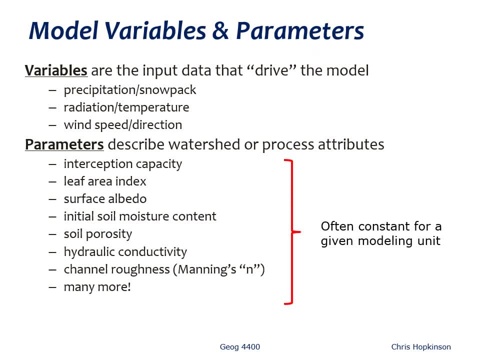 can be negated if data do not exist to adequately set up or run the model. Once a model has been decided upon, we need to collect the data to set up or parameterize and to run performed simulations with the model. Variables are the input data from which runoff and. 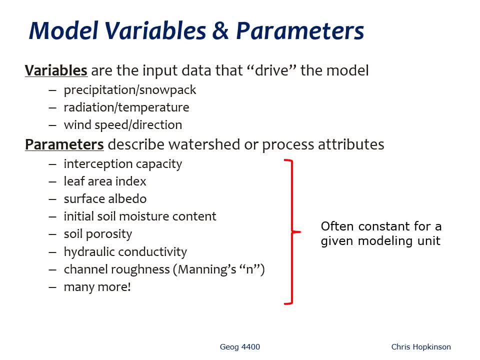 or evaporation, etc. will ultimately be calculated. Parameters tend to be fixed or quasi-fixed numerical descriptors of watershed attributes that influence the way inputs are transferred through or lost from the watershed on their way to the outlet. Scanning this list of parameters, you'll probably note that some clearly are not going to be fixed. 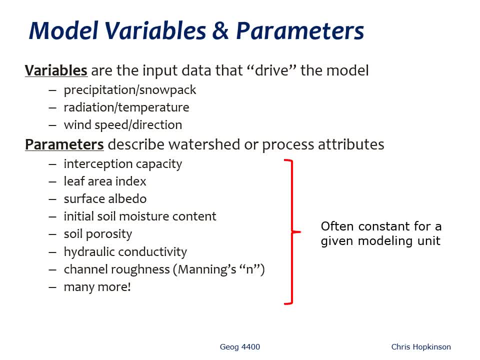 For example, leaf area index can vary by a great deal over the course of a year. So if your watershed also displays such variation in vegetation cover, then your chosen model must accommodate time variant parameters. Some models can do this and some cannot, so herein lies one of the challenges of modeling. For pragmatic purposes, we sometimes 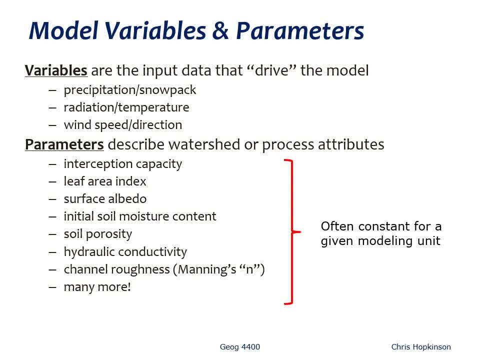 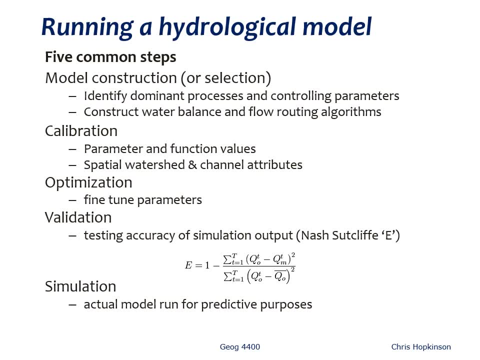 have to assign fixed parameter values, but in reality, the world is more dynamic. Okay, so now we know something about the principles of modeling and different types of models, but how do we go about setting one up and running a simulation? Well, that would be too much to go through in detail here now, as there are lots of 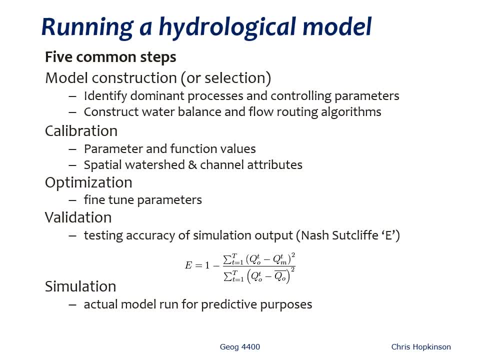 off-the-shelf models to suit many different hydrological conditions and scenarios. However, in general, we can use the principles of modeling to set up and run a simulation. We can also use the principles of modeling to set up and run a simulation. However, in general, there are five major steps. 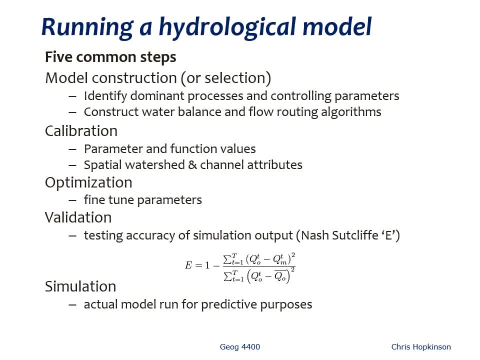 Depending on the nature of the hydrological problem you wish to address, you can either select a pre-existing model or, if your problem is unique or does not require a complex model, you could create your own. For example, simple models can be constructed in numerical and spatial. 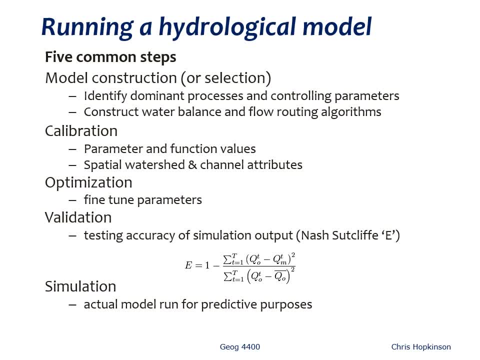 analysis packages such as Microsoft Excel and Esri, ArcGIS, Or, if you're quite brilliant and have lots of time on your hands, they can be coded from scratch. Once a model is in place, the simulation requires four further steps. The first step is to create a simulation model. The simulation model is: 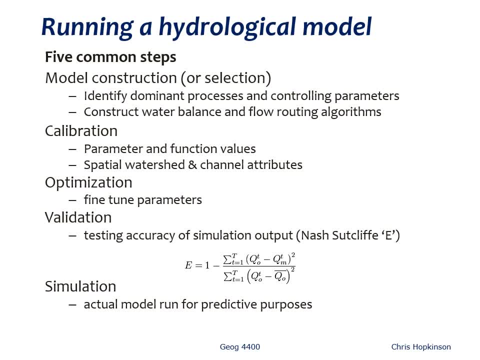 the first step to create a simulation model. The second step is to create a simulation model. Calibration, parameter optimization and validation are often interrelated and even iterative steps to ensure the best possible modeling conditions. Once we are satisfied with the model setup. 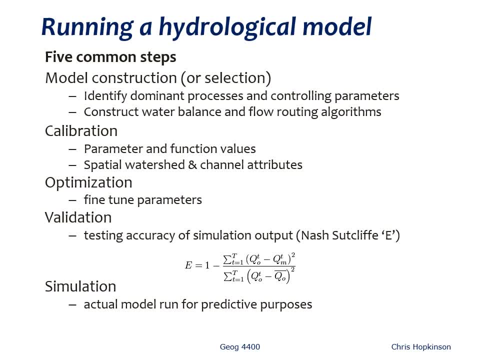 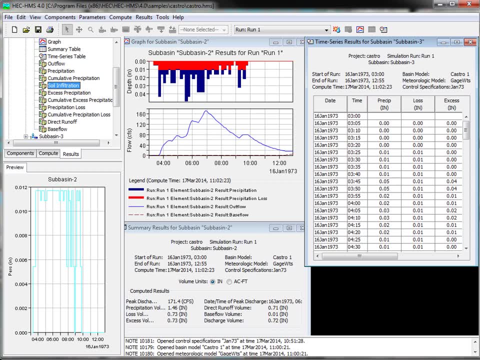 we can then perform a model run or simulation of the scenario that we wish to evaluate. As noted, hydrological models come in various forms, but here is one example of a modeling interface. This is the freely downloadable US Army Corps of Engineers Hydrological Engineering Center Hydrologic Modeling System, or HEC-HMS. 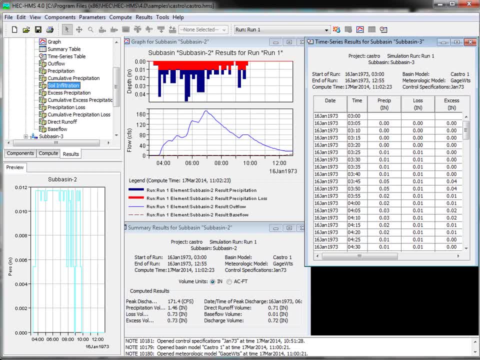 On the left, we see the model, component or object manager, as well as a preview of sub-basin precipitation input data. In the center, we see the time series, plots of precipitation, the associated loss and the output hydrograph, along with some summary data describing the event. 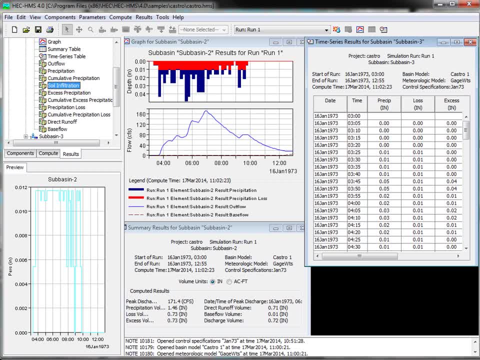 being simulated, And at right we see the numerical data associated with the plot. Many other windows can be entered within HEC-HMS for model setup, simulation and reporting, and all models will have their own particular interface style. One element to note here is that the discharge is 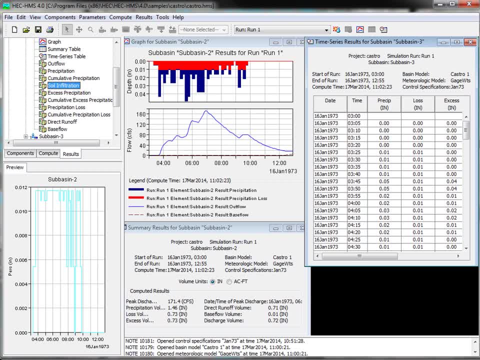 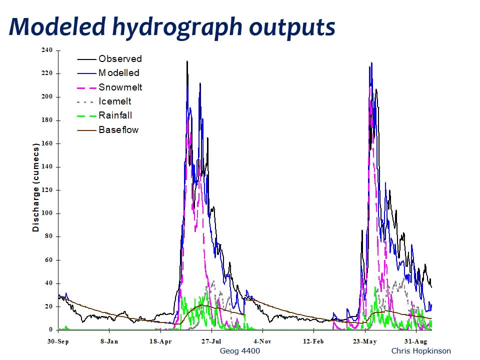 presented as a total runoff hydrograph and no partitioning of the flow is illustrated. Some models will produce outputs of runoff as well as water balance partitioning within the hydrograph, as we can see here as an output from the UBC watershed model. 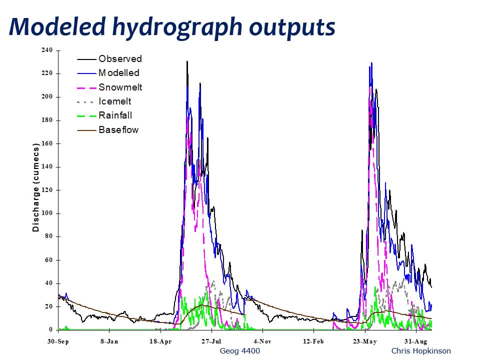 While this might represent the endpoint of a hydrological model, this is often the starting point of further analyses, such as flood inundation modeling or decision-making processes. The example here illustrates two years of simulation on the Bow River upstream of Banff, Alberta, in the Canadian Rockies. In this case, the question being asked 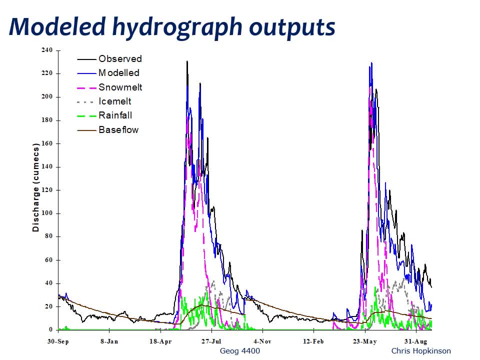 of the model was: how important is glacier ice melt relative to rainfall and annual snowmelt runoff? Overall, glacier ice melt produced a similar amount of runoff to rainfall, but only a fraction of the snowmelt proportion. Snowmelt is a dominant runoff component on the Bow, as it is with most rivers in this region. 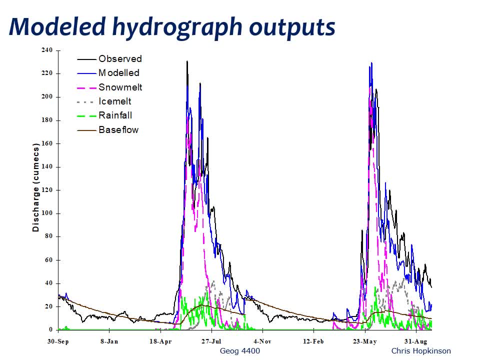 However, the glacier ice melt fraction is critical, as the timing of peak ice melt production occurs when snowmelt and rainfall inputs are reduced. Thus, ice melt elevates flow levels in late summer, when the resource is most needed for human and ecosystem services. 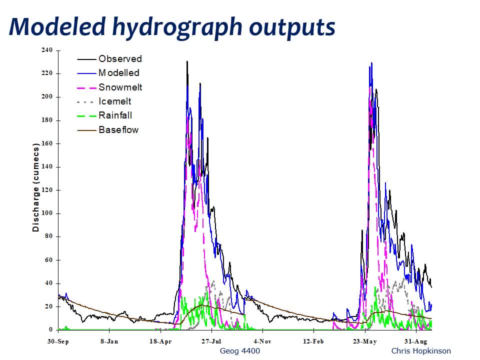 This has potentially serious implications, given glacier ice is reducing throughout the Rockies, While we are able to make observations of glacier recession and runoff. the overall hydrology of these basins is complex, with many inputs and outputs. Therefore, we need models to make connections between the many inputs and outputs. 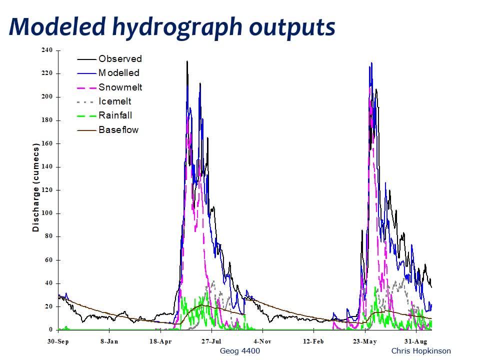 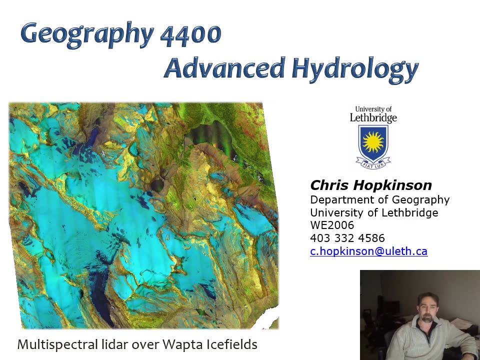 and to better understand the system. With the enhanced understanding that models provide, we are able to gain knowledge about processes, locations and times for which we cannot make direct observations. Well, thank you for your attention and I hope you found these slides informative. Chris signing off.